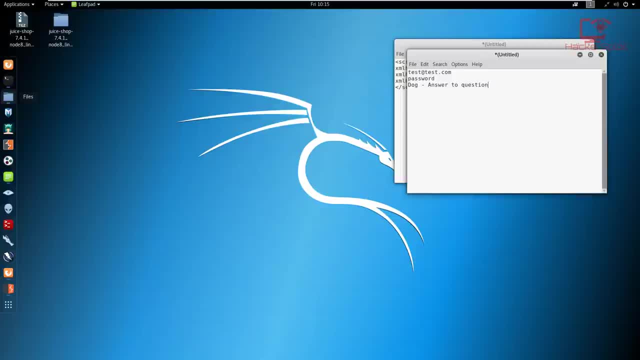 correctly. So, for the purpose of this video, I've set up a very unique environment that in- at least in my opinion, will demonstrate how to utilize or how to perform this attack. Alright, now I'm just going to give you a brief overview of the environment that I have. Now, of course, you can 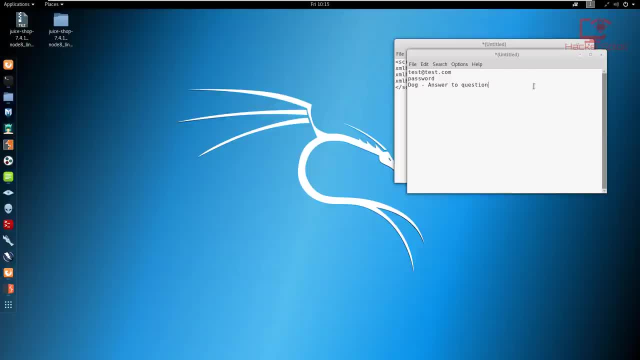 see, I have a few files open here. Don't worry about them right now. Just just remember that we'll be using them later on And I'll be using them really, really well to explain what's going on here. So you can see, as my target or as my vulnerable system, I'm going to be using my 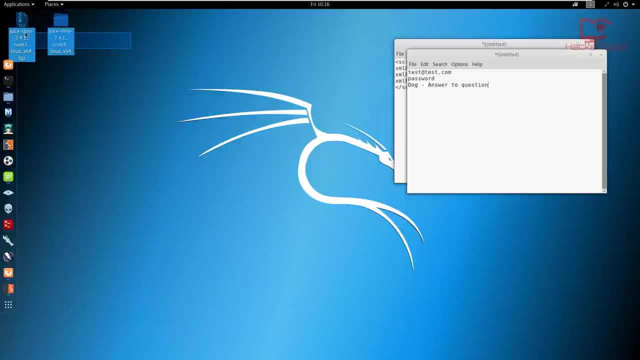 vulnerable web application. I should say I'm going to be using the OS juice shop Now, not actually. no one actually recommended this to me, But I remember that I performed this during a CTF challenge that I went to earlier, I think late. 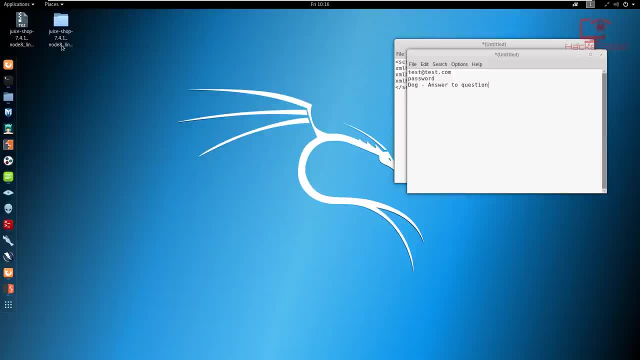 last year- I'm not too sure exactly when, but the whole process was involved with exploiting this web application All right, And in my opinion this really outlined or really showed off how to perform all of these various web application attacks In this case. 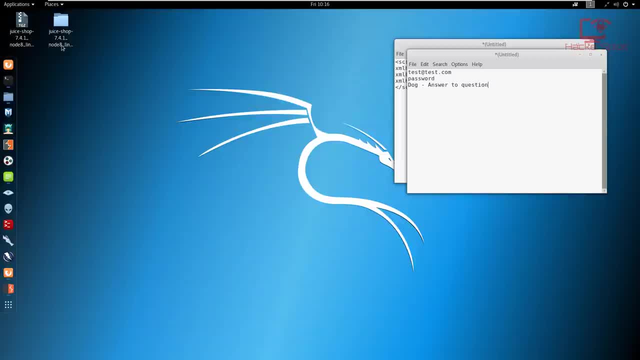 we're going to be focusing on cross site request forgery. Alright, so I have the juice shop running. It's. it's based on nodejs And it's running on my localhost. Let me just show you that right now, There we are. So I haven't logged in or done anything yet, And that's because I'm 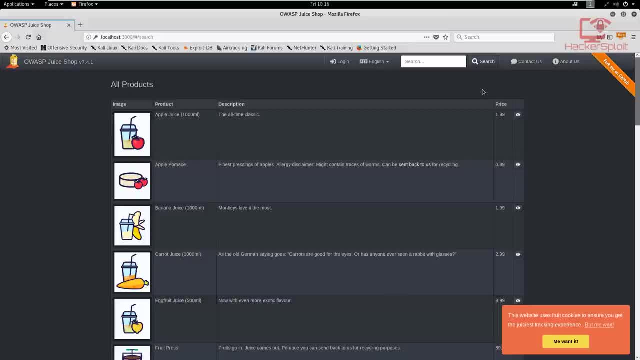 going to do that with you, So I've set it up. it's running on my localhost. If you want me to make a video now to set the OS juice shop up, I will make it, because this is a fantastic way of explaining how everything works and understanding how these attacks work And in 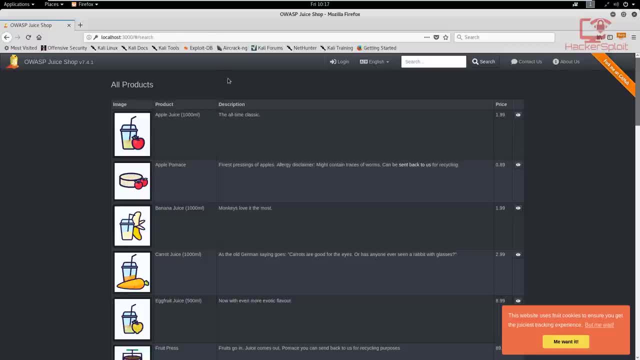 regards to that, the OS juice shop is a complete CTF challenge that you can run or take place in or you can. you can go through it And if you find the flag well done, So remember. if you want me to make a video of that, just let me know in the comment section down below. So let's get started. 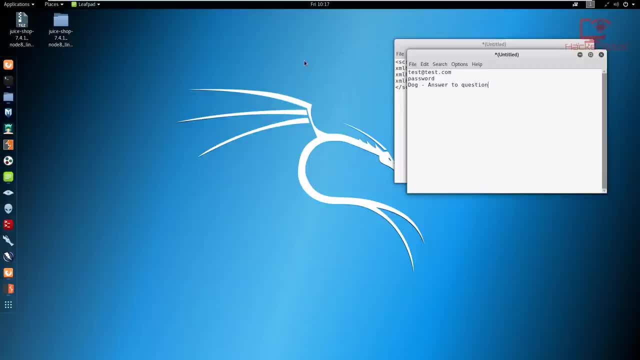 with this really really simple but sometimes complicated topic. Alright, so cross site request forgery- CSRF. Now, from the name you can already tell that it's it into two, into two sections. you have your cross site and your request forgery. So from 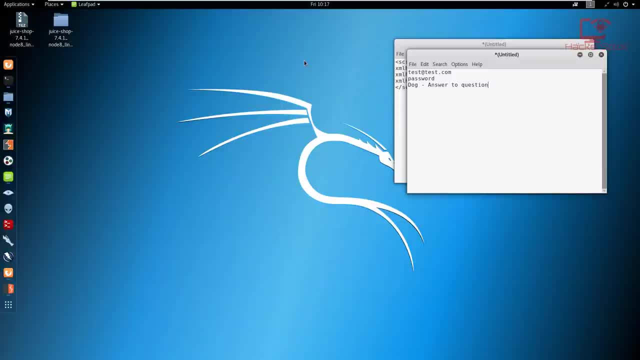 that we can get a basic example of what's going on here. we have cross site scripting and we are going to be forging requests or we are going to be manipulating requests. Hmm, interesting. So we are. we are kind of understanding what's going on here Now. 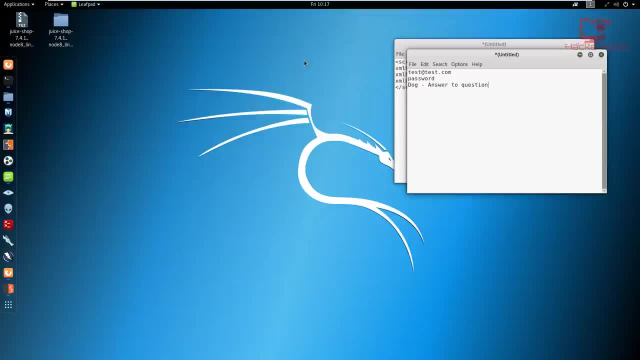 the technical explanation for what CSRF is is. it is an attack that forces an end user to execute it unwanted actions on a web application in which they are currently authenticated. Alright, so let me put that really, really simply right. it's an attack that will force an end user to execute unwanted 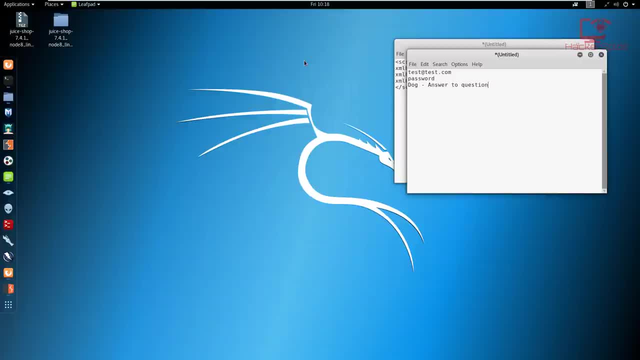 actions on a web, on a web application. these actions can be anything, But in this case we're going to be looking at changing the password And they have to be currently authenticated to that web application, which means they have to be logged in to that web application for this to work. 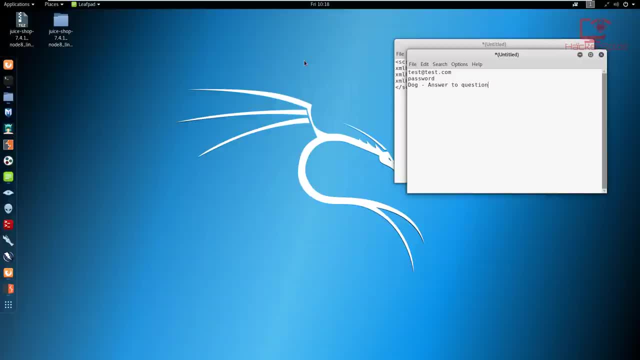 Because if they are logged out then you get the idea it really doesn't help or it doesn't work. Alright, so we use cross site scripting in this case to perform the request forgery and to get either desired or undesired. 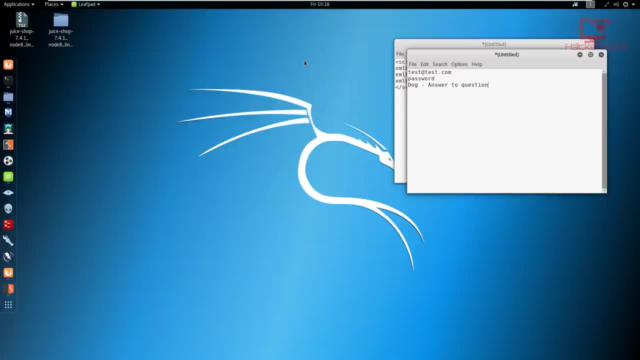 results. In our case, we're going to be looking at how to to change the password of any user that's logged into the to this web application, And how will we? how will we be doing that? Well, we are going to be using CSRF, But the first thing you need to understand is how an HTML form 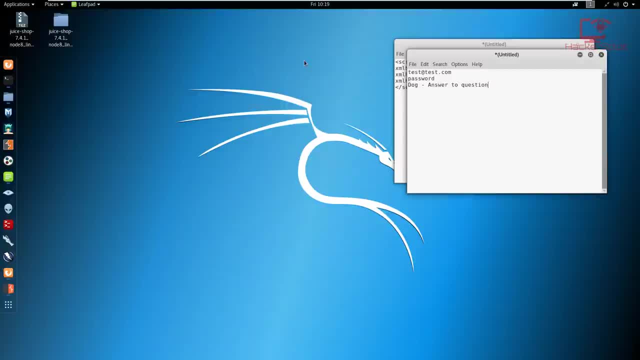 works All right, And this is very important because, first of all, a client will request a page from a server, All right, the server will then respond and give the, the client, the HTML form. the client will then send back the, the form with the data back to the server. 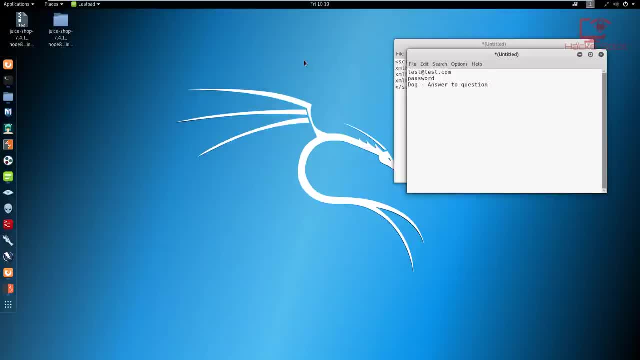 the server will then authenticate and authorize the user and then will will perform the requested action And, based on the request and the response, we are able to forge or to change the request. So request and get a desired response. if you're looking at it from an attacker's perspective, 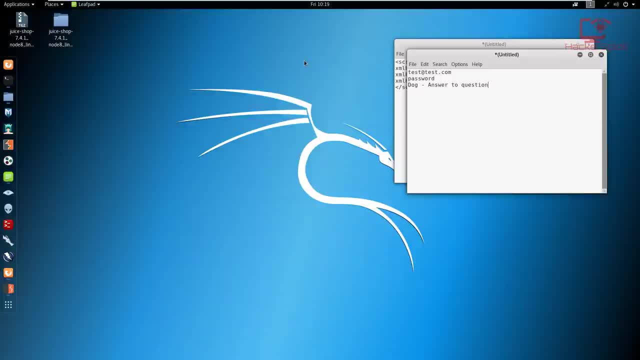 Alright, so the the way CRS, CS, CSRF work- sorry about that- is the attacker will manipulate the victim into submitting the attackers form data to the victims web server. essentially, essentially performing these, these requests. In our case, as I've mentioned, it will allow us to: 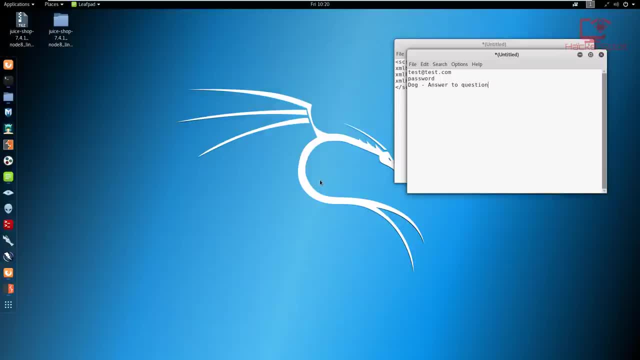 change the password of any user on this web application, In this case the OS juice shop web application. Alright, so now you might be asking: well, if I'm a bug bounty hunter or I'm practicing to become a bug bounty hunter, How do I go about finding this vulnerability? 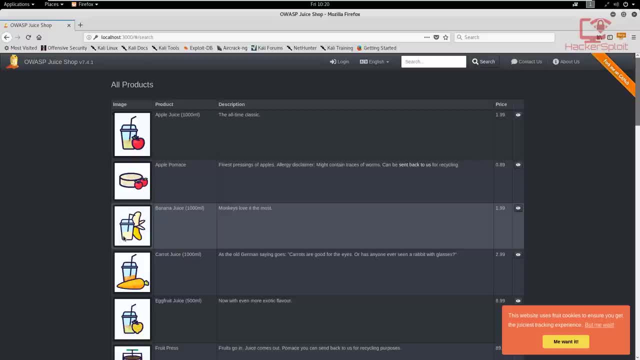 Well, that's a very good question And that is the question you should be asking yourself when performing any penetration test. Now, coming back to my environment, I'm running burp suite, the Community Edition. you you'll just need the Community Edition For this one. we're not. 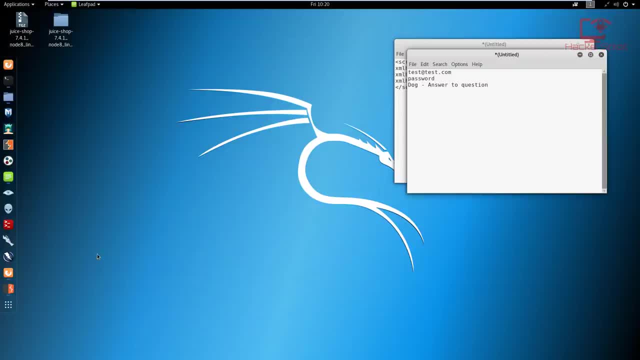 performing any advanced penetration. So in this case, what we're doing here is we're taking a techniques here, because we're essentially just changing. we're just going to be changing the request to get our desired responses, But once we move on to the advanced stuff I'll then be using 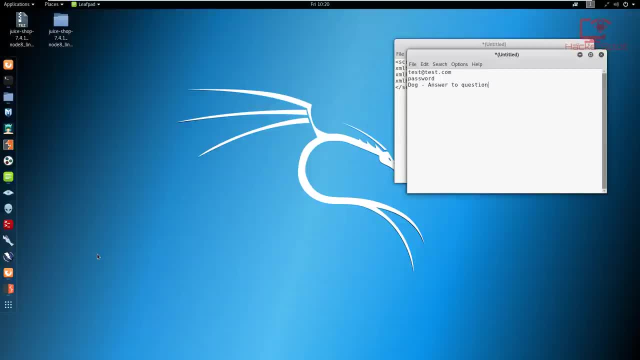 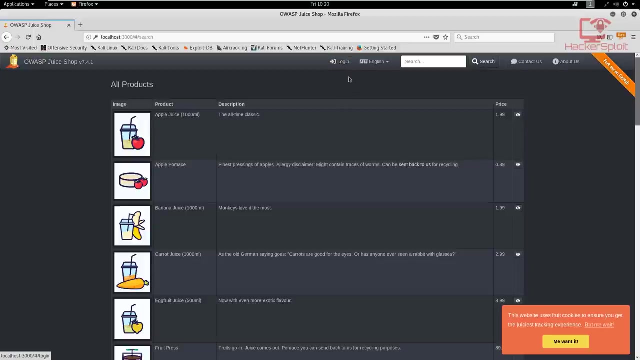 OS zap for our attacks. Alright, so, keeping things really, really simple, we the way to look for these vulnerabilities is to target the login pages, which we have right here. we then need to. we can then create the account and log in, And then, finally, we will be creating our own, our own. 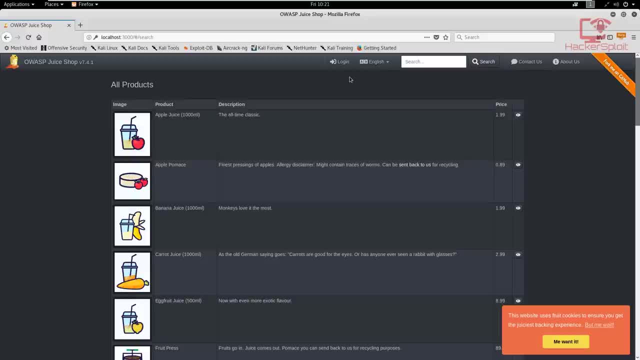 script to perform the cross site scripting And that will allow us to submit the data. or, if we send the URL to another user of this web application who is currently authenticated, it will allow the. it will allow us to make them change their password And then we can log into their 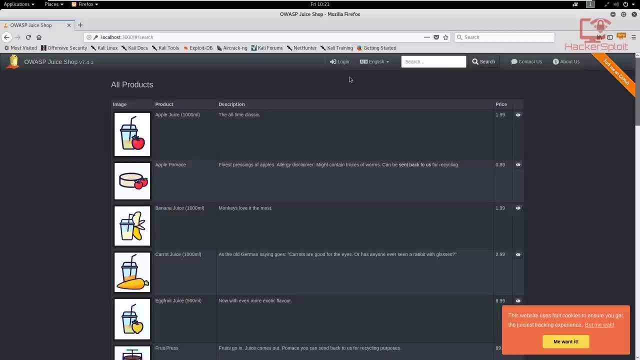 account Alright. so this vulnerability is very common on sites with accounts. you know, sites that have email addresses And then we can log into their account, And then we can log into their emails passwords And, as you probably would have guessed, there are a lot of sites that utilize. 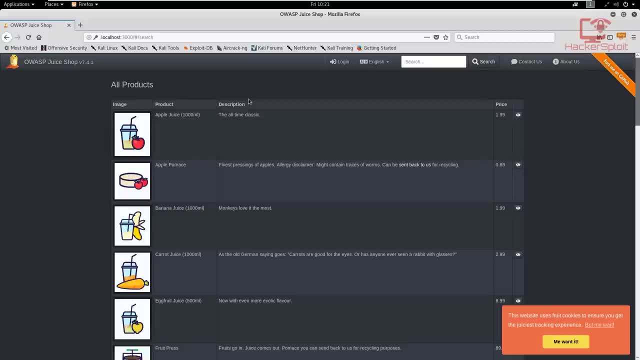 this functionality, But remember, most of the sites out there will be protected from this vulnerability, So it's up to you to find these vulnerabilities. Alright, so, as I've mentioned, we will be using OS juice shop as our target, And the reason is is because it will explain. 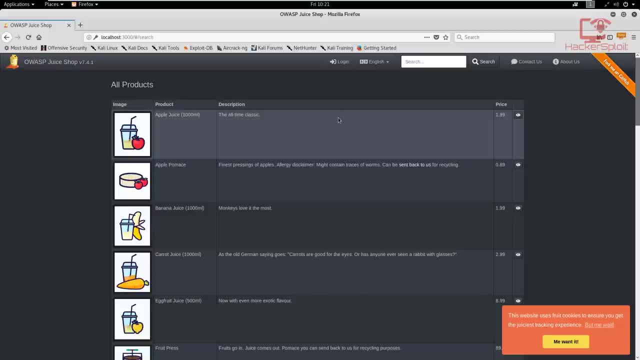 what I want to explain. really, really well, Alright, and we'll be using the burp suite Community Edition. Now, as you can see, I'm currently running the burp proxy. I'm not intercepting any traffic if I open a burp suite. I'm not intercepting any traffic if I go to the. 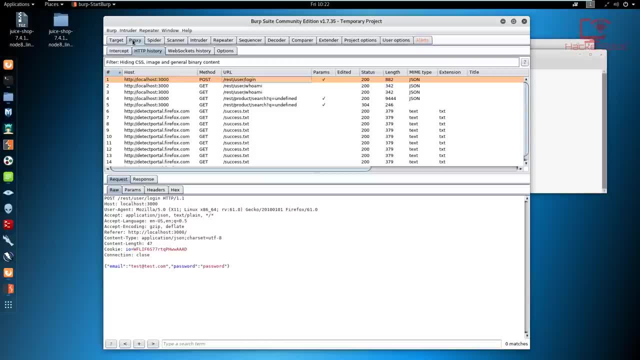 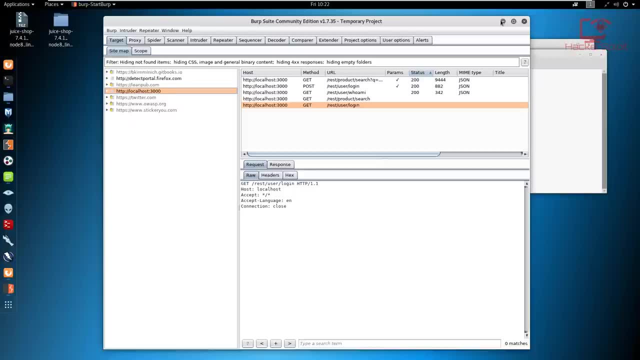 proxy and intercept. I'm not intercepting anything, So it's currently just I'm just going through the burp proxy and all traffic and data is being logged through the burp proxy. So when it comes down to this little data that I've saved here, I've already created an account. 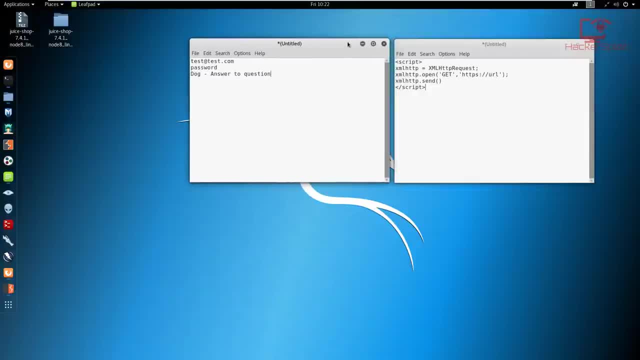 the reason I've done that is to save time, because I don't want to explain everything about it. So I've created- I've created a user with the email of test at test calm and a password of password. So really simple. Again, there's nothing really complicated. 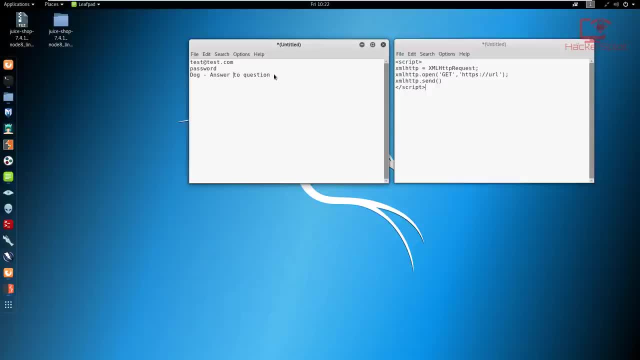 here And, if you want, if you're wondering, what exactly does this mean? Well, this is a security question with the answer. So the the question was: what's my favorite pet? and I wrote in dog, So hopefully that doesn't scare you into thinking that I've gone completely crazy. And then in here. 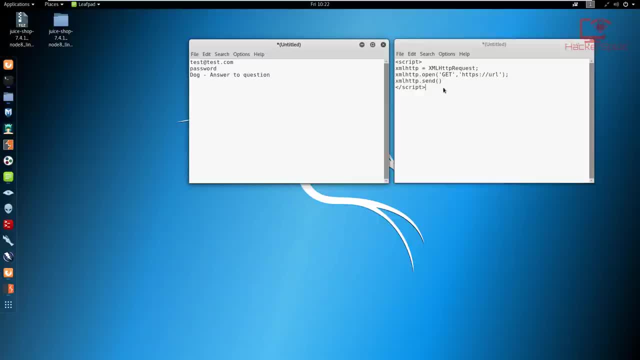 we have the script that we'll be using, or we'll be utilizing, to perform the CSRF on the site. I'll get to this in a second, So let's go ahead and start this. So let's go ahead and start this Second. we don't need that right now. So if I want to log in, I know that the the email is test. 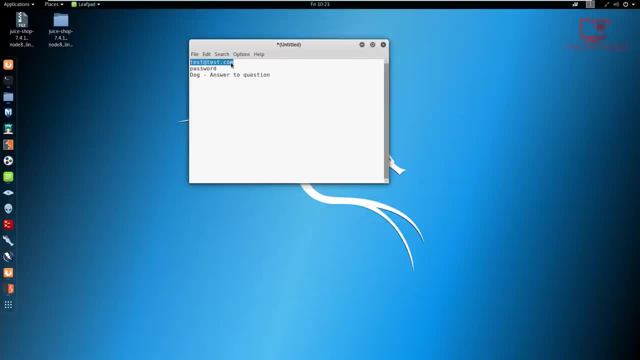 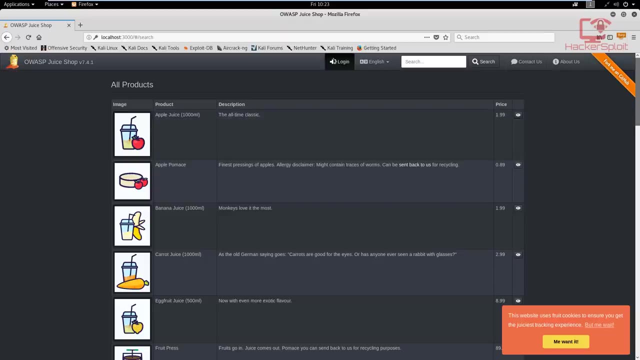 at testcom And the password is password. Alright, so let me do that. right now we need to authenticate, So let me log in, like so, and I'm going to hit test at testcom, Alright, and I'm going to write the password, which is password, and I'm going to hit login: Alright, and I'm don't. 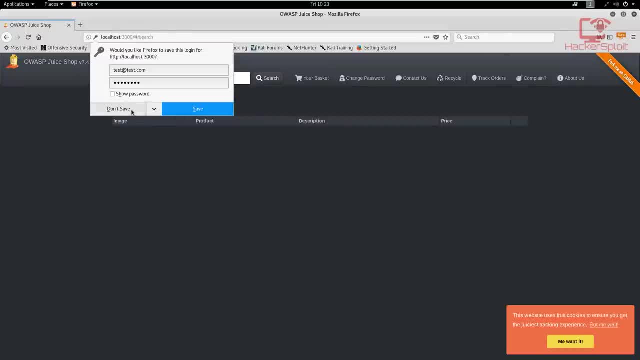 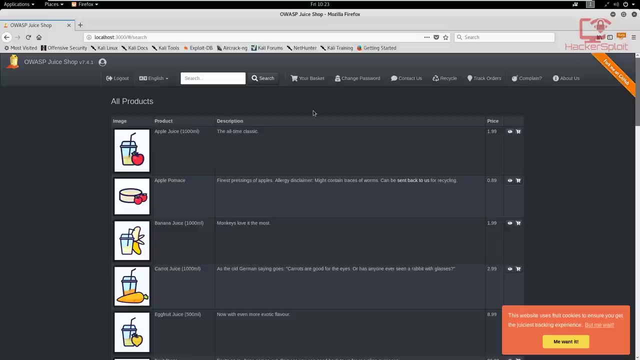 want to save the password And there you are, So I've logged in now. Now, as I said, this is very. this vulnerability works really, really well when you're talking about changing passwords because, as you can probably guess, an attacker 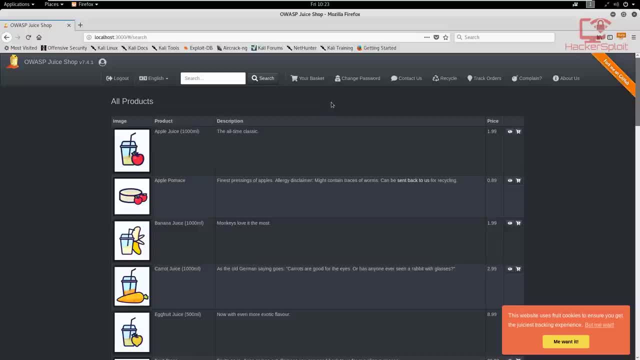 would would be looking to exploit this functionality Because imagine if we were able to send a request to get request to our target with the URL encoded URL. of course, we can also use link shorteners if we wanted to do that And, essentially, if they authenticated it. 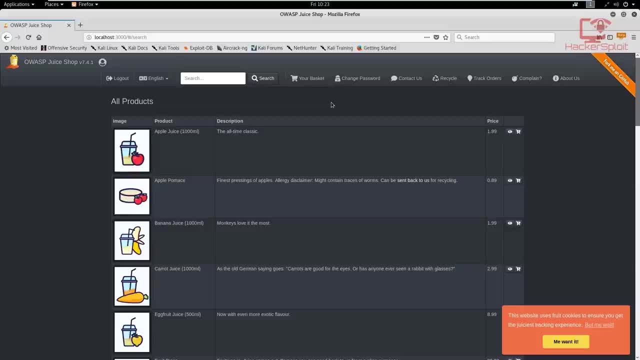 it will allow us to make them change their password simply by clicking on the link changing the password to whatever we specify. Alright, so how do we do this? Well, the first thing to do is we need to look at how the get requests are being sent, And we can do that using 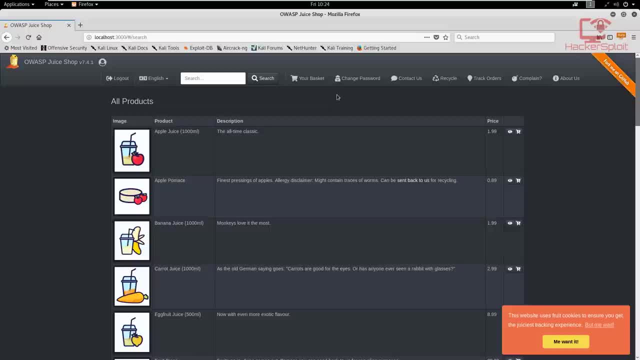 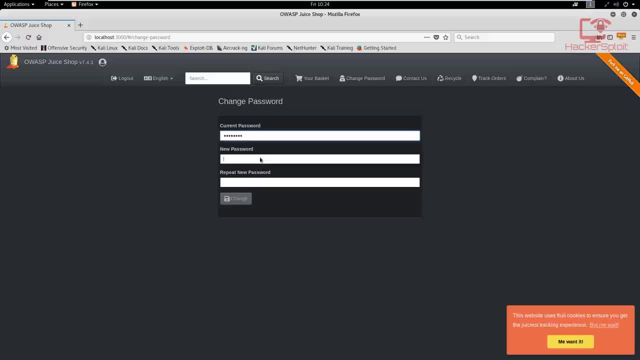 burp. So we are just going to change our password. So our current password is password And what I'm going to do is I'm going to change my password into password. Oops, sorry, pass word 123. And I'm going to repeat it. So pass word 123. And I'm going to hit change Alright. so the password was. 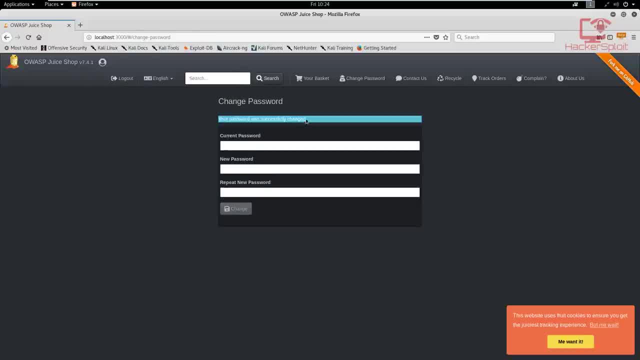 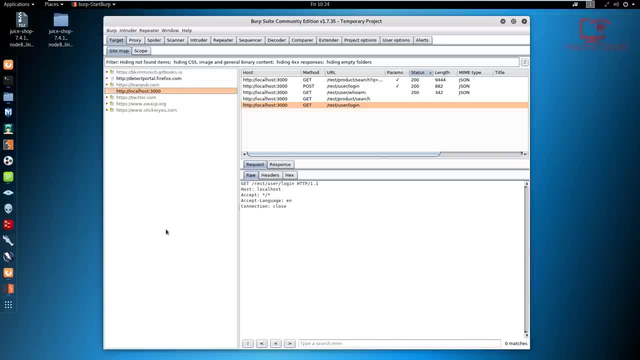 successfully changed. Okay, now let's look at how this was changed. So let's look at how this was processed in burp, or how the request was sent in burp. So I'm going to go into burp proxy and HTTP history And I'm going to go all the way to the bottom And, as you can see, we have the get. 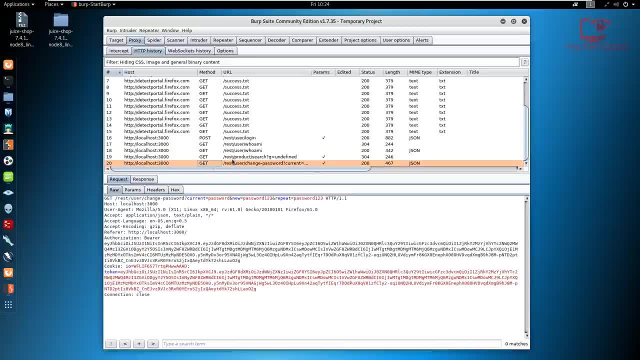 request right over here. Okay, so the get request is very interesting. you can see we have the get request and it's targeting the. the following URL And these are the parameters. So change password. the current password is password new password: 123.. And we've repeated it. Alright, so now let 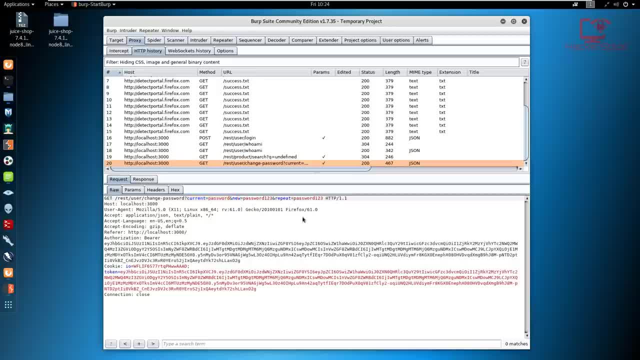 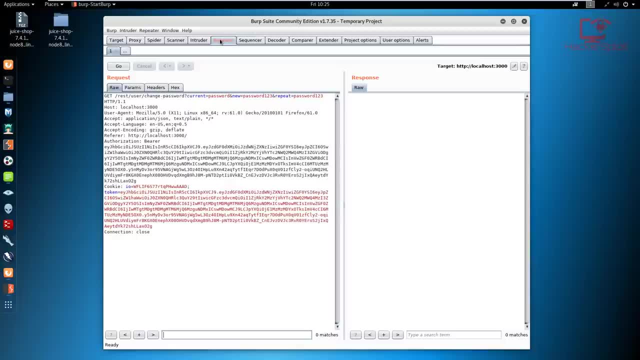 us perform the forger Here. So I'm going to send this in to the repeater. Alright, so I'm going to click on repeater And in here we can manipulate the requests and see what responses we get. Alright, in case you you did not. 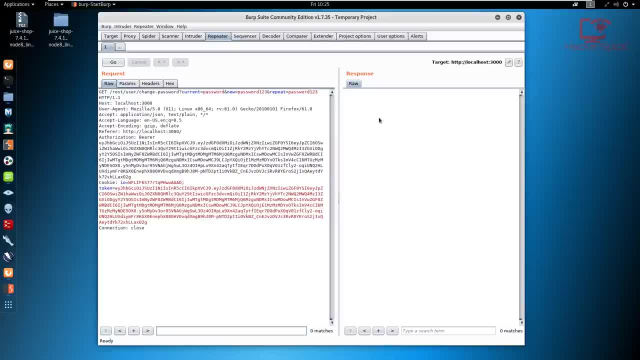 know about that. But again, let's start off really, really simply. So we are going to be working with the raw request. we don't want to work with individual parameters- although you could change it- but we are going to be manipulating the request entirely so that it performs what we want to do. 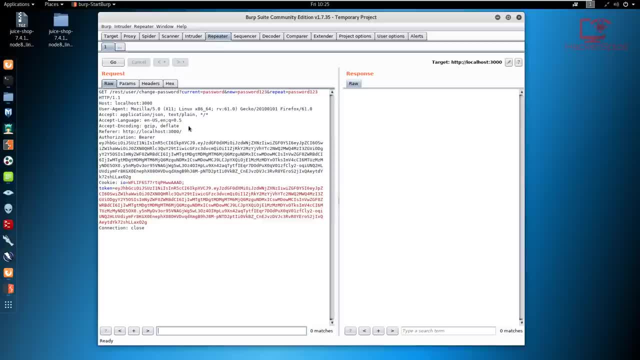 Alright, so what we can do first is: we can test, So let's change. what if we were to change the current password to something like: let's see, test, let's change it to test, And then we hit go. you can see that the response we get is: 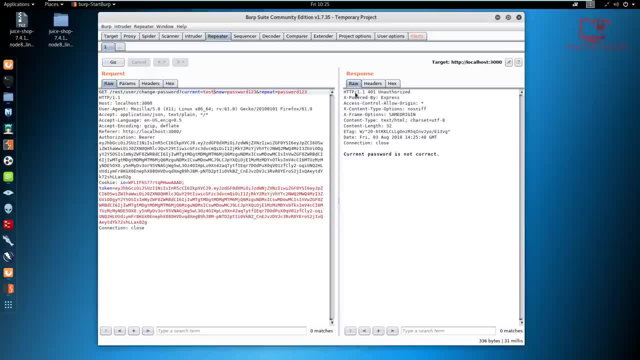 a is a 401 error, which means we are not authorized to make that, and it will give you the message right here: The current password is not correct. Alright, that's good. That is good from a web application perspective, which means that this web application is performing validation And it's not going to. 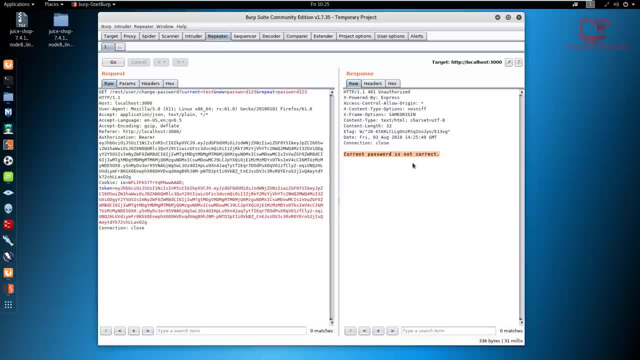 you know, to just go in and start manipulating any requests and making changes. So, from a security perspective, the web application is doing really, really well. Alright, what if I was to change the new password? Let me change this back to password, to the current password, which is what we set, And 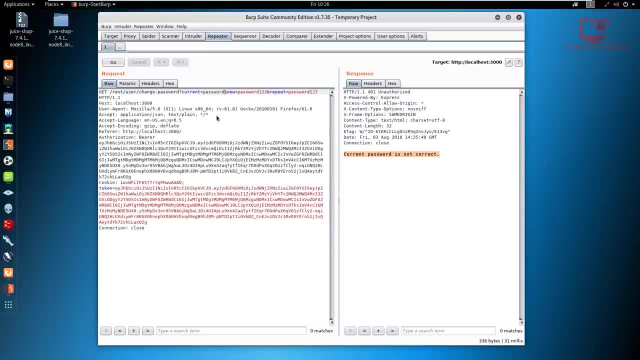 I changed the new password to password pass 123.. All right, and I hit go Again. we get another error And again the 401 unauthorized error, Telling us that the new and repeated password do not match. So yes, the current password is correct. 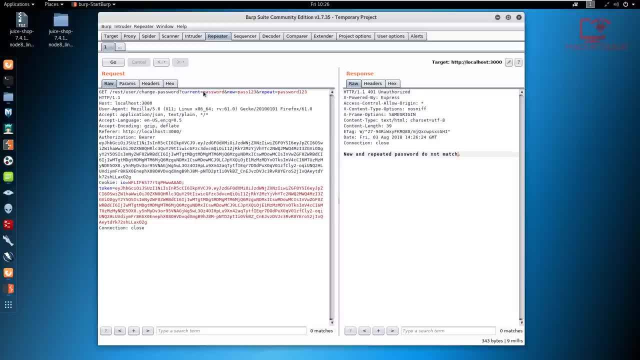 And the only thing that we're getting an error is the new password and the repeated password are not correct. So interesting, what if we want to change the password into password 123. And we can repeat that again? So we want to confirm this, or password 123. Actually, hold on. So I'm going to say: 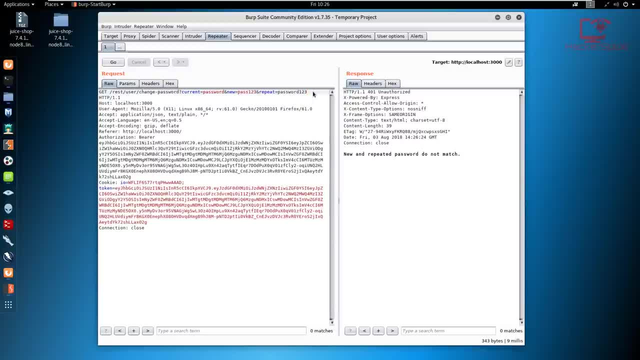 password 123.. And now let's see what this tells us. this should verify it, But let's see if this works, So you can see. yes, that does work, And we know that this works because that's what we did. That was the original. 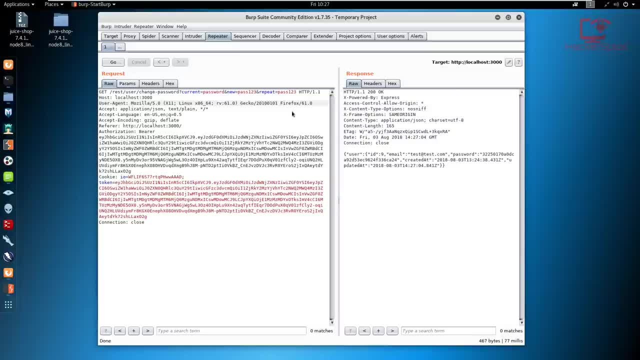 request. But what if we do not know the current password of the user? Remember, we're going to be targeting other users of this web application. So what if we get rid of- and this is very, very this is the way penetration testers go about it- What if we get rid of stuff? So what if we get? 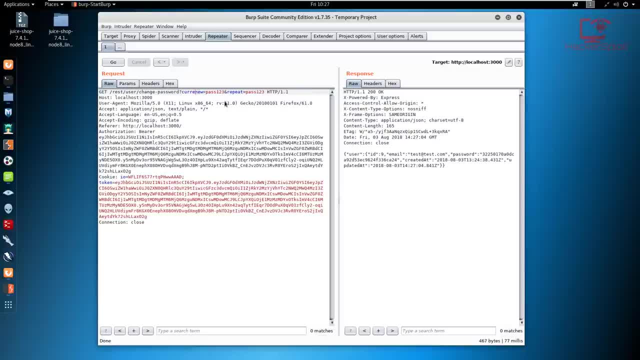 rid of the current password, Alright. and now essentially the get is targeting change password, with the question mark here essentially requesting- and we only entering the fields or parameters new- and repeat: what if we do that and we change them to password 123. I mean pass 123 and pass 123. 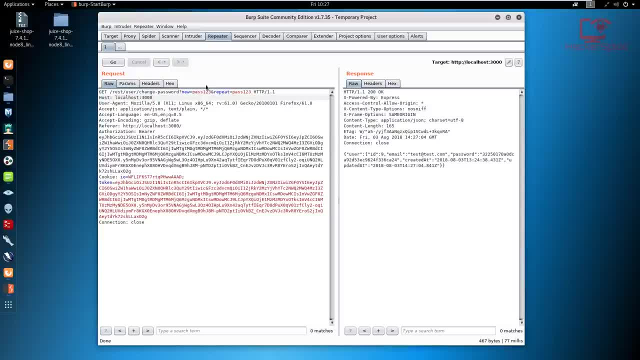 Let me go, you can see. yes, it does work. We get the 200. The 200 response, which means everything was processed correctly And we were able to get a password that looks to be hash, that looks to be hashed, And we got the email that we use. So, yes, we do know that it is. 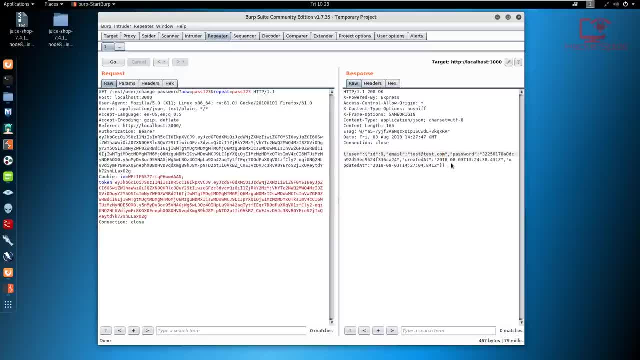 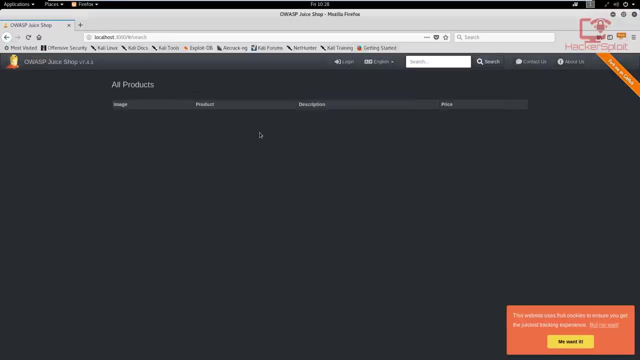 working Alright. so we know that. we know that this worked. but we need to confirm that this has worked. So we can do this by going back into our web application And we can log out and we can try and log in again. So log in with our new password. So we're going to say: test at testcom. 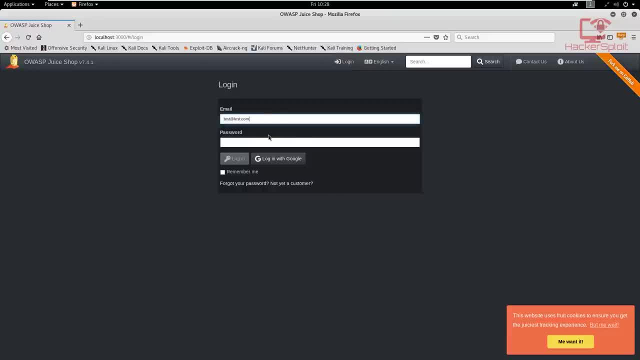 And our new password was pass 123.. Remember we changed it earlier. But again, I was demonstrating that we, if we are to send this to our target, we need to specify to make sure that it will work without any pre required information, like. 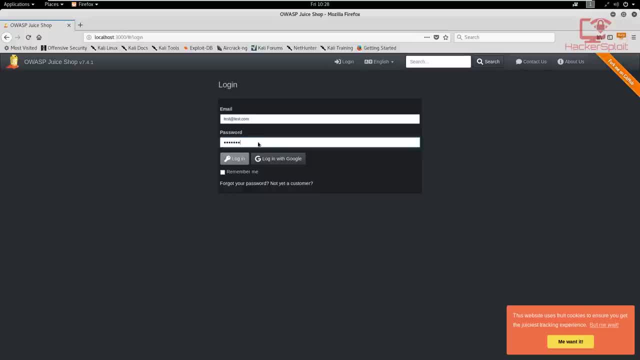 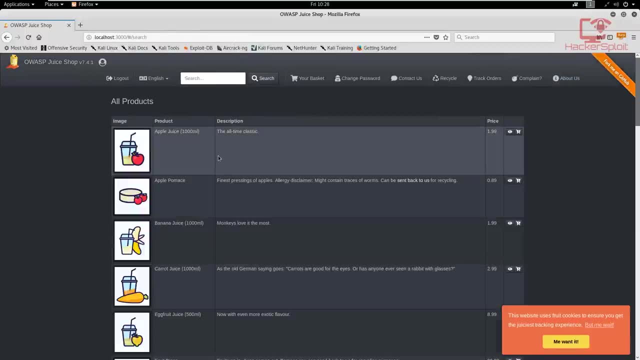 their current password. So we've manipulated the request there. So let's hit login And voila, you can see it does work Excellent, Alright. so this is a fantastic example of all CSRF can be utilized, or how it can be. X, how you can find vulnerabilities for it. Alright, so this can allow. 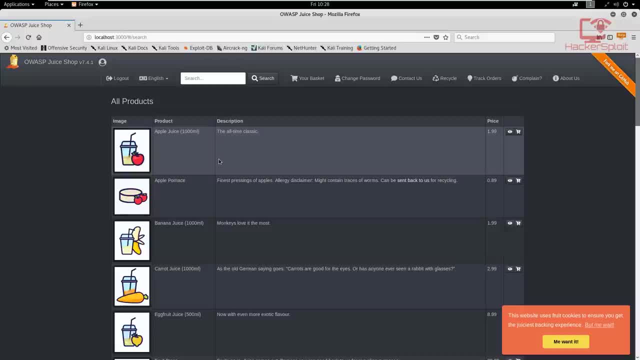 us to change or upgrade Anyone's password, anyone's accounts password that are currently logged into this web application. Alright, so now? what do we? what we need to do? Well, we can. we can log in, As we've already seen. 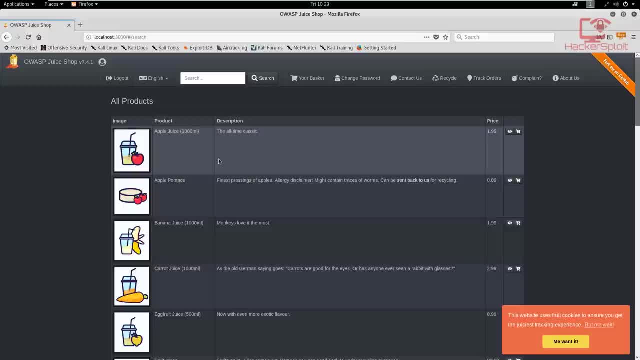 we can log in And once we've logged in we can, we can test to see if cross site scripting does work, And then, of course, utilizing it throughout the web application is very important. So we can run a simple cross site script attack to see if it will work on the search bar right here. So I 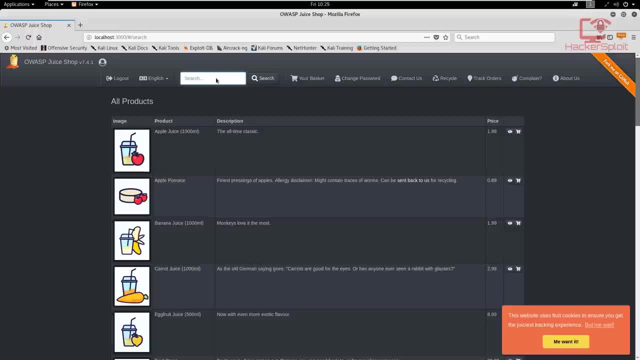 am going to type in script and a simple one, So alert, just to test whether it works, And in the alert we can say: Hello, just something stupid, Hello world, you know that's, and I can't even. 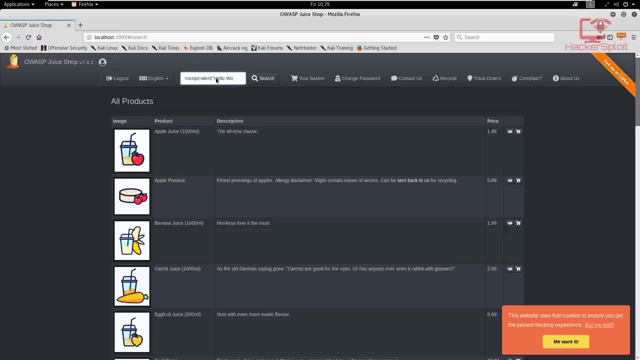 type: man come on world, And we have typed in the alert and we can finally close the script here. Script like so And let's hit search And voila, we can see that, indeed, cross site scripting what works, which means we can insert. 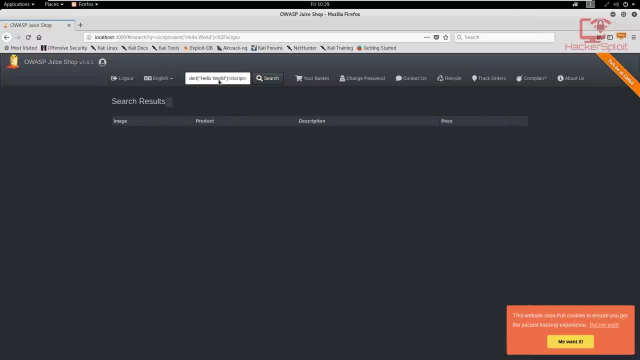 we can insert our our get request inside a script and and use a cross site scripting to perform the CSRF, And now you can see them conjoining together cross site scripting with request forgery. Okay, so we now need to create our custom script that will allow us to utilize the attack, And we will 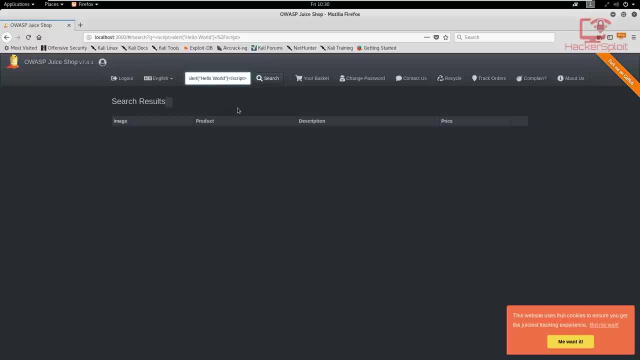 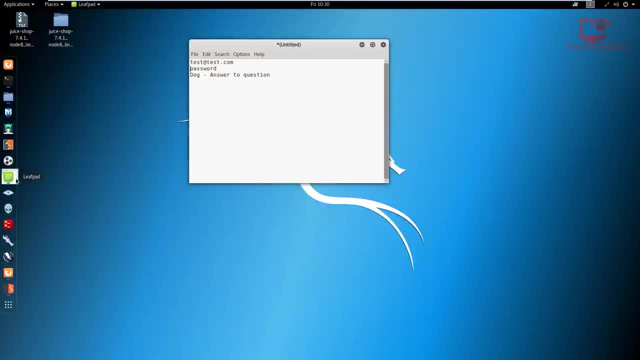 be using XML and HTTP. Now you might have seen this script right over here. let me just minimize this and open up leaf pad. you might have seen this script that I created. Now you can find many of these CSRF scripts on the web application. So let's go ahead and create our custom script And 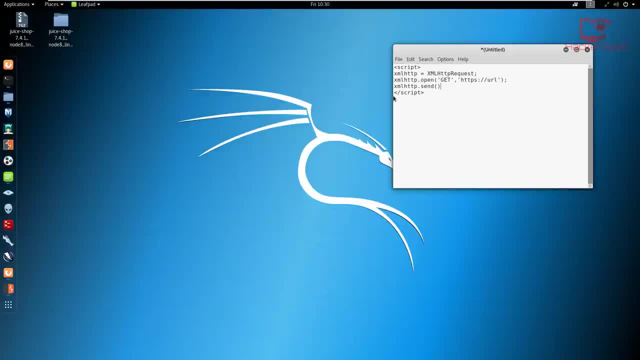 we're going to use the get request, And we can see that we have a few of these. we have a few of these different languages. In my case, I find the one that works the best is the is the one that works with x, xml and HTTP and contains the get request in here. Okay, now you can see that the get 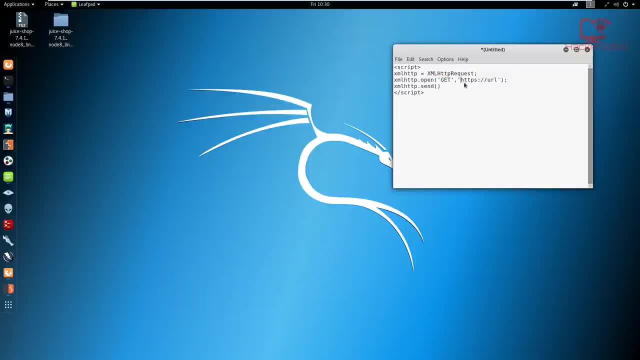 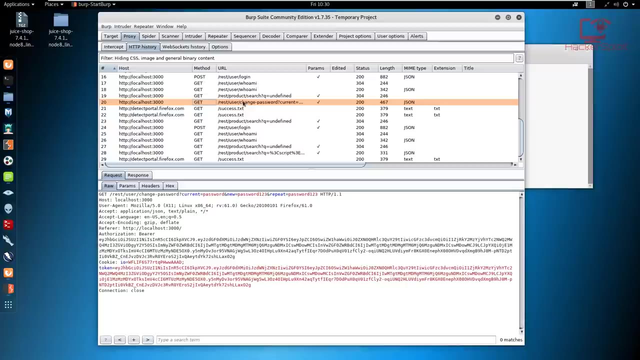 request requires the URL in which we submit the parameters without the current password. So we need to go back into BEP And if I was to go back into proxy HTTP, sorry about that HTTP- we look to change the password there. So if we go back into- sorry the repeater and if we look at 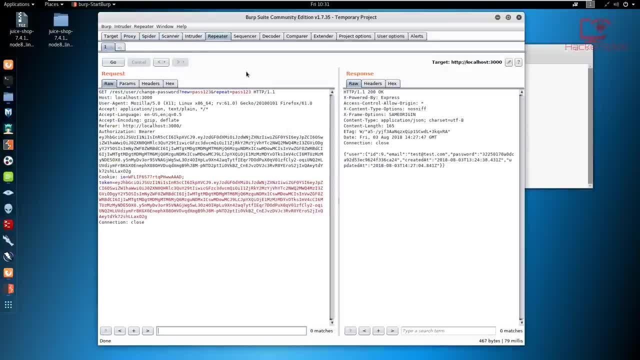 this. now we can see that the URL is right over here. So that's the get request. So if we copy this, the localhost obviously, and we are not using any current password field. So if we can do that really, really simply, you can see how this can be utilized really really well. So. 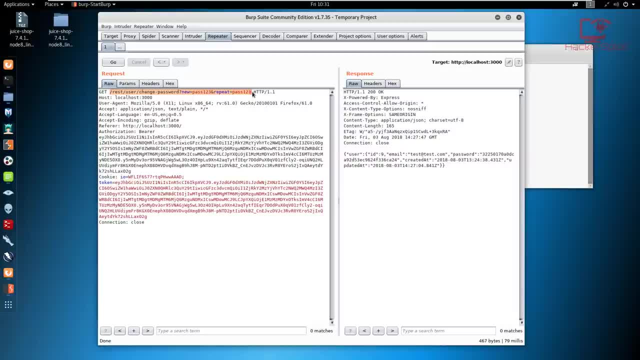 what we need to do now is understand how the URL will be formatted And, of course, the web application is going to encode it- and I'll get to that in a second- So we need to copy this URL right here. So I'm just going to copy the URL And we can edit our, our script. So HTTPS and we. 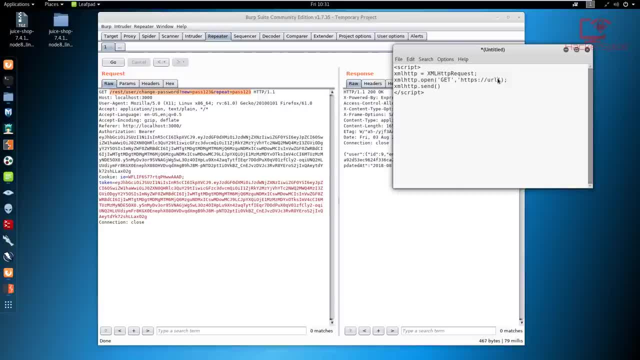 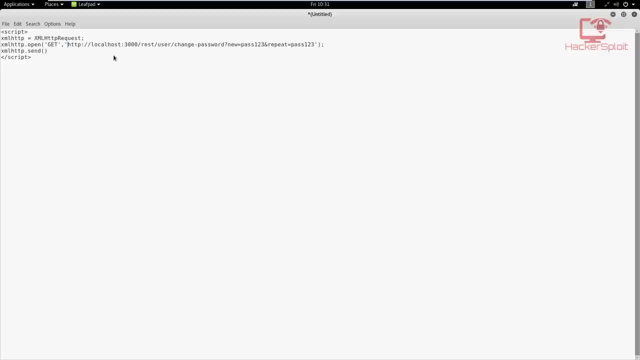 paste it in inside the URL. you can copy this script if you want to. Let's take a look at whether this script is formatted correctly. So get HTTP. No, that's not the way we want it. Let me get rid of the pre predetermined HTTP there. So HTTP localhost. it's hosted on my localhost with. 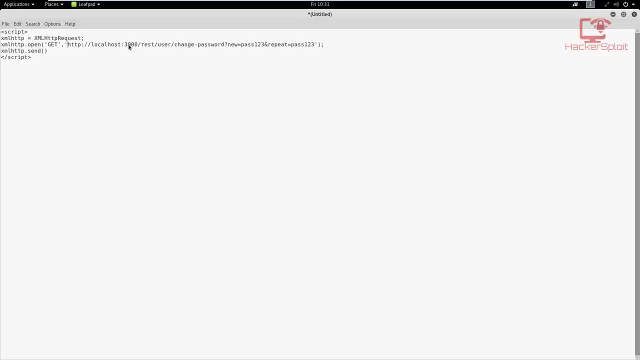 port 3000 node, node js standard And the. we want to change the password. the new password is pass 123 and repeat is pass 123.. You can change that to whatever you want. if you want to, you know, play around with the script, But in my case I don't want to do any of that. So this is the. 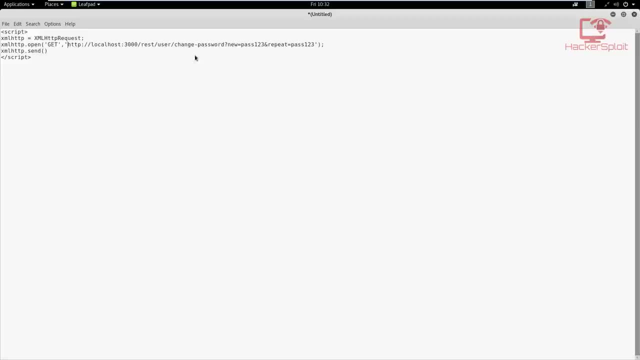 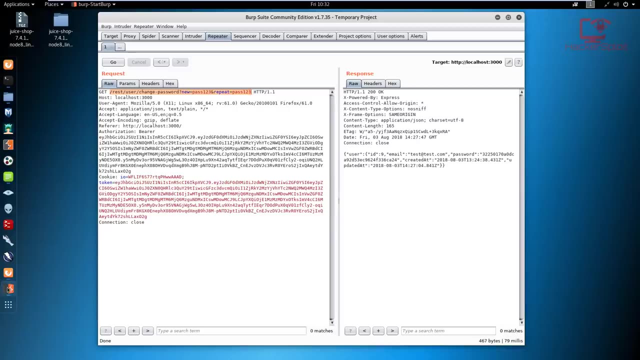 script. So what we can do is we can copy this now And we can run this in the search bar, And that should, in theory and in practice, give us our first CSRF attack on the site. So I'm going to paste this in here And let's see whether it does this. 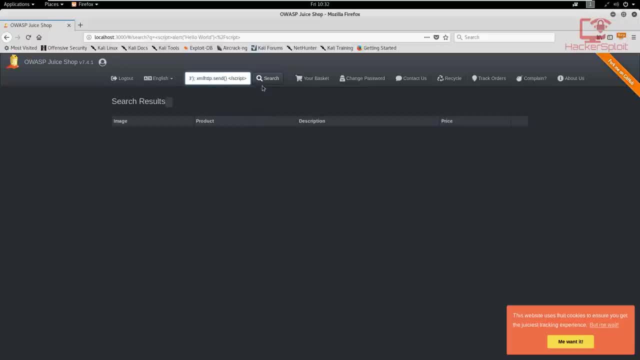 So I'm going to search And you can see you successfully solved. solved a challenge, error handling provoke, an error that is not very gracefully handled. Again, this is a fantastic web application: vulnerable web application that is awesome for practicing your, your web application. 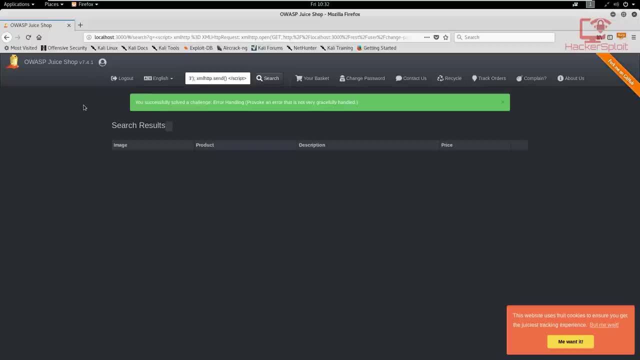 penetration testing skills. Now, I talked about the URL that you should send to your target, And that is the URL that will essentially make them change their password, or, without them knowing, given that they are logged in to the web application or they have an account. it will not work if they've not logged in. Alright, 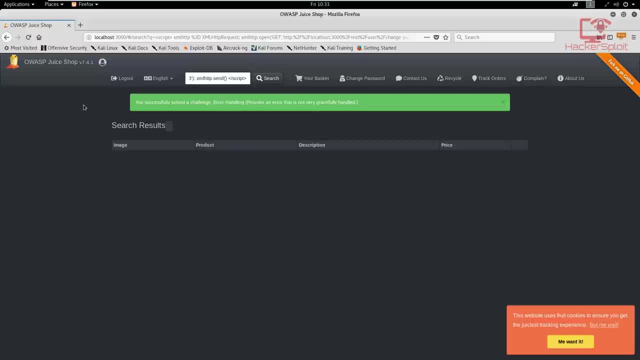 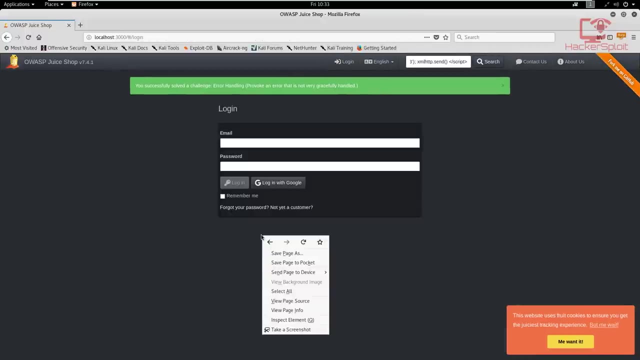 so that's very important to understand And many people, just you know, forget about this. Now, Again, if you could have done this, you, I can log out again and I can log in. try and log in now And I can type in, for example: test. I just want to show you something very interesting here: test. 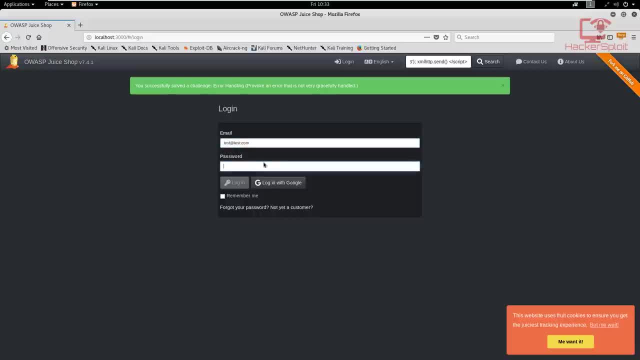 and I can change the password. we already changed it to password 123.. Now, before I do that, I can just inspect the element here And I'm going to hit login And I just want you to check something out. Alright, now let me just expand this a little bit here. If we were to look at the 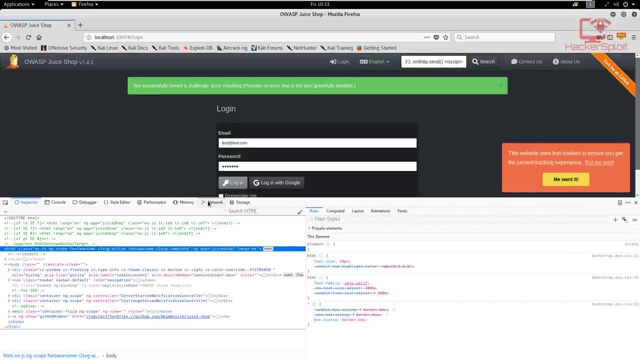 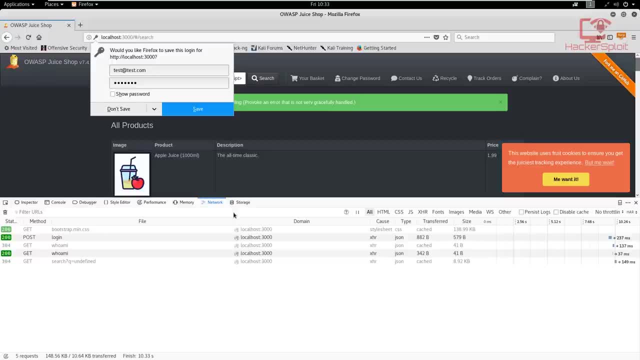 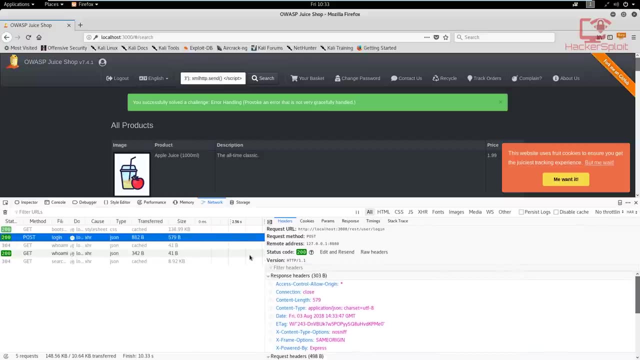 network. this will essentially show us all the get requests. So if I was to hit login, you can see that if we are to look at the get request here, the login get request, you can go ahead and look at at the, the exact format in which it was sent. you can look at the cookie, the. it should give you the. 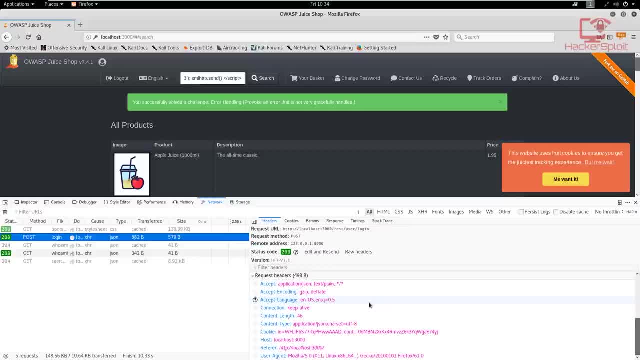 authentication token. not to show it should give you the authentic, the authentication token, But that's something for another day. I don't want to complicate you guys. you can look at the cookie if you want to, And you have all the responses right here. So there we are. there's the authentication. 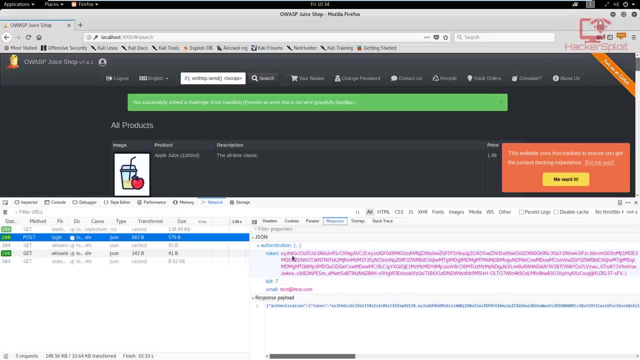 token And you can see something very interesting in regards to the token. Alright, so let me show you this right now. Alright, so, as I was saying, you can see. alright, so, as I was saying, you can see that if we look at, 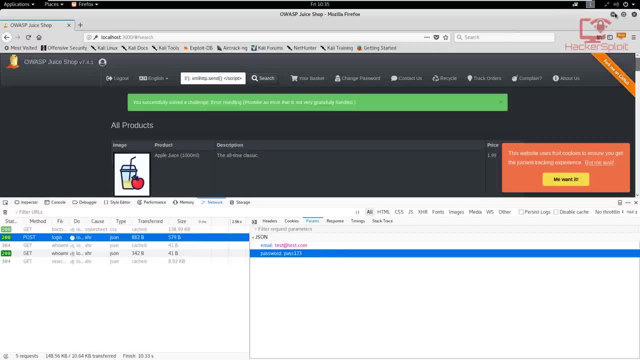 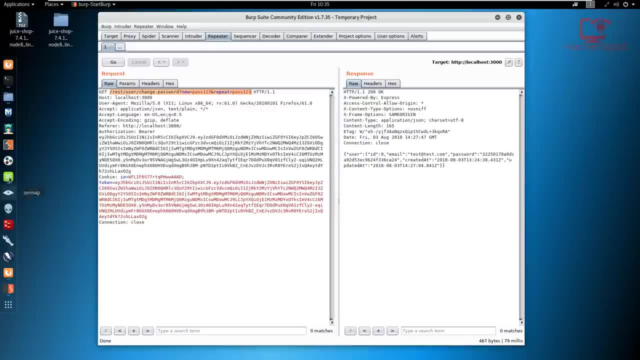 the parameters. the password will be displayed there and it will be updated to the one that we selected or specified in the script. Alright, so remember, if you want to customize the cross site scripting attack, you can do it through your script. And where is leafpad here? So there we. 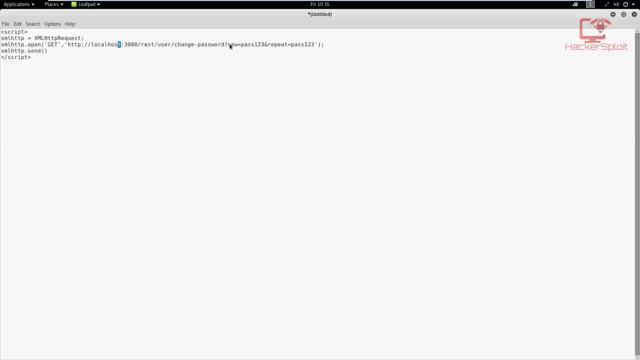 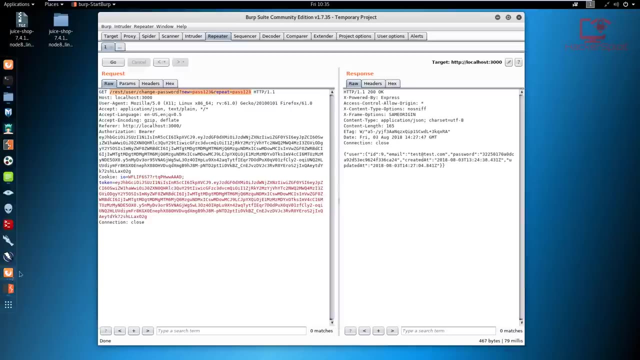 are. So you can change the password, the. as you see, we just got rid of the current password parameter, which is a one vulnerability on the site, but you can change the password to whatever you want. And now you might be asking, as I've mentioned, what link do you send to the target? And that is very, very simple. 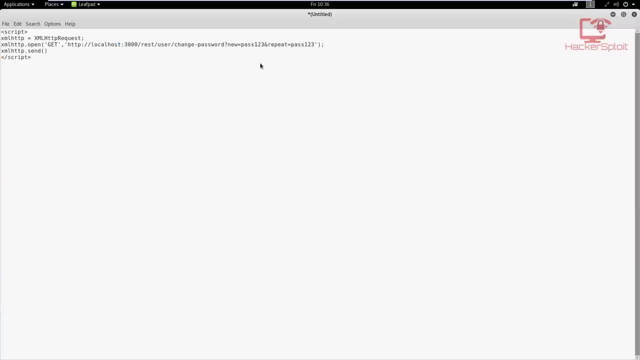 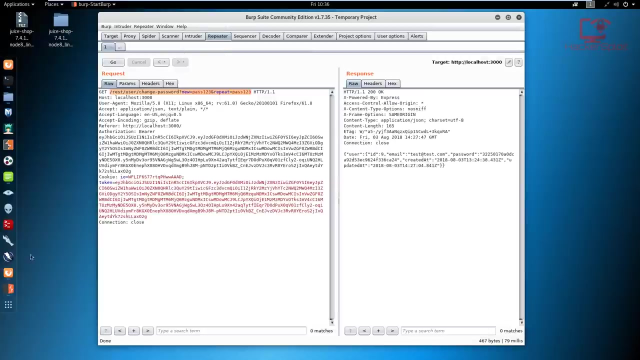 If I was to run the script again and I changed the password to maybe something else like a password 124, or 345.. Sorry, three, four, five, let me just add that to the password. And I run the script on an authenticated user, which is me. So let me copy that And it should change my. 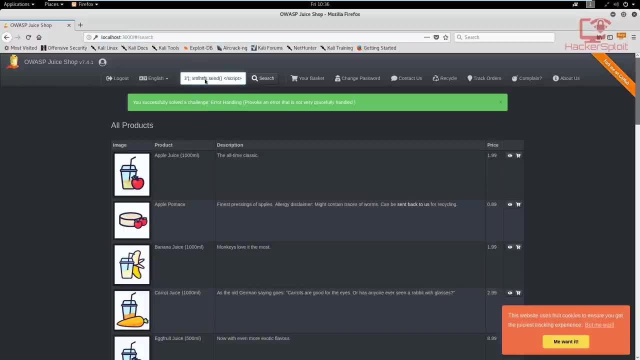 account password And you can see, once I log out, log out and try logging in, it will have changed it successfully, So let me just run it in here. So I'm going to paste the new one in here And I'm going to search. 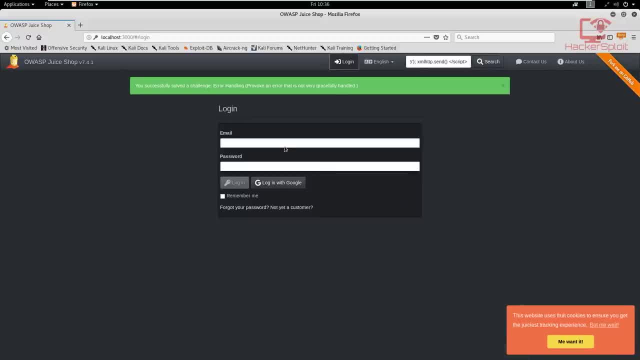 and there we are. So now it's changed my password And if I log out and I try and log in with with the old password, which is password 123, you can see? whoops, sorry, I think I typed that in wrongly. 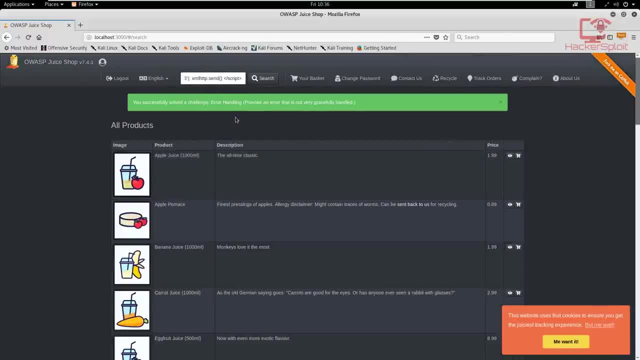 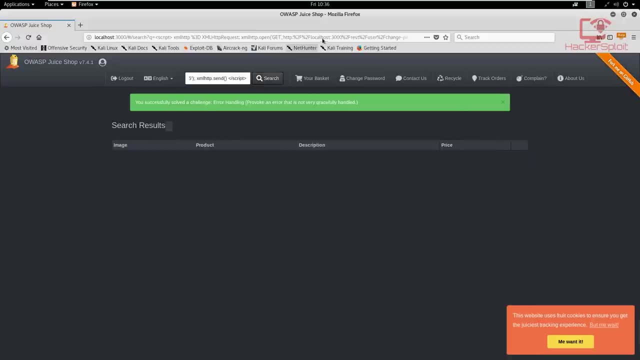 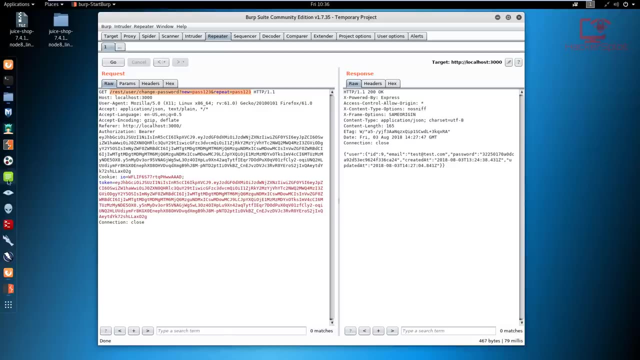 123. Like. so fight, login. There we are. you can see that we entered the new password and it did work- Fantastic. So we were successfully able to execute the script. And again, when? if I just run the script again, this is the URL that you will send to your target. Alright, so if I just copy it and I 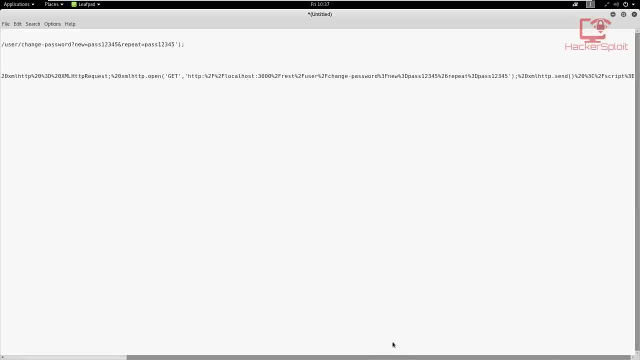 inspect it in my leafpad here. I really love leafpad. I don't know that you guys love it too. if I just inspect it, you can see that this, indeed, is a URL, And if the web application was being hosted on a server outside my local air network, it would give you the website name, the port, if it. 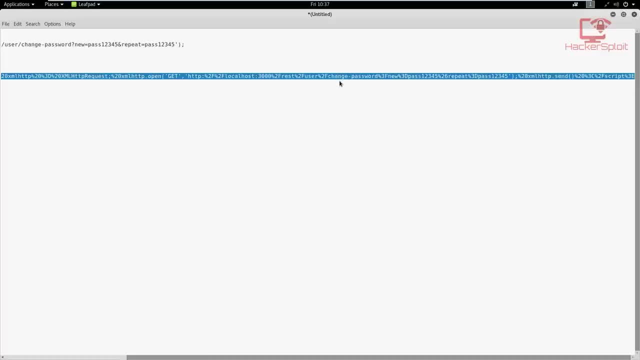 is port specific and the URL here. So that's what I'm going to do, So I'm going to go ahead and here, which, as you can see, is encoded, So what I would recommend. So what I would recommend is that you copy this link here and you use a link shortener like 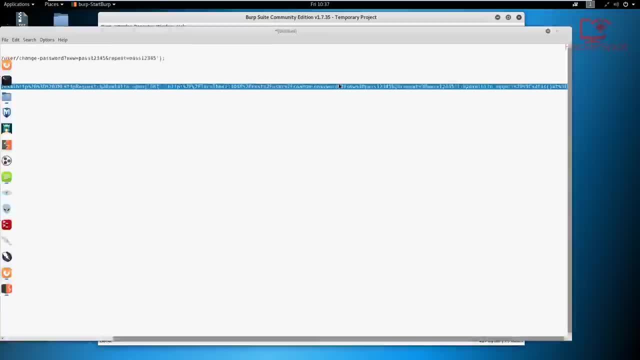 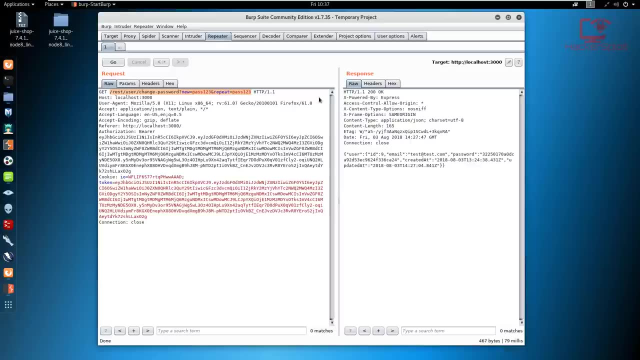 bitfly or any of the other Google shorteners, and you send that to your target And once they click on the link- and if they already logged in to this specific web application, it will update their password and you can. essentially, you have their password now because you've updated it And you. 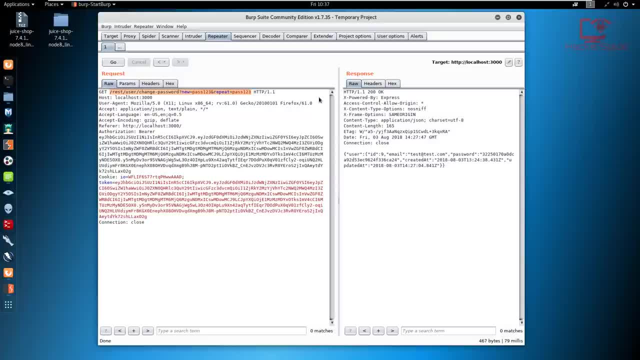 all you need is the email, which I'm pretty sure you must be knowing if you're performing this attack, Or you could just be gathering passwords of users or of which you can. you can send this link to and are authenticated with the web application. Alright, so that was a very advanced. 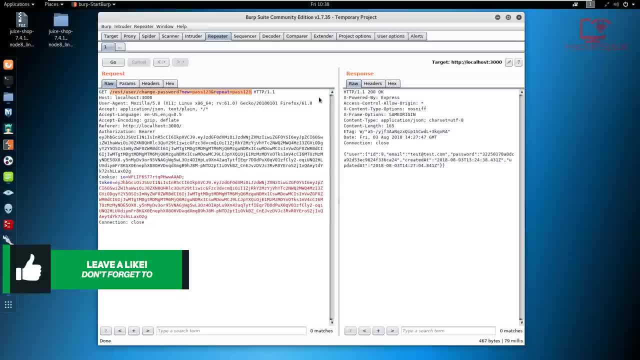 topic that I wanted to explain And hopefully I was able to do it using juice shop. So, yeah, that's going to be it for this video. guys, If you found value in this video, please leave a like down below, If you have any suggestions, questions or anything else that you would like to ask me. 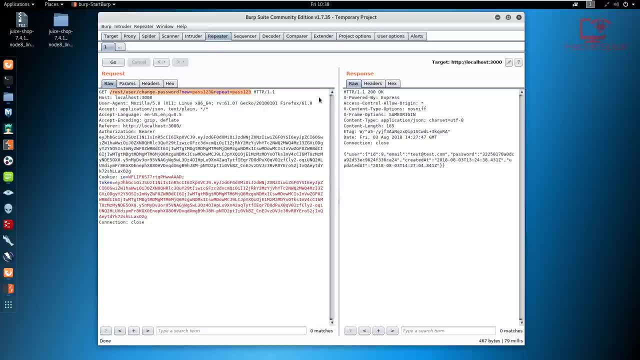 leave them in the comment section on my social networks or on the website. If you want to support the channel, you can do that by clicking on our Patreon. the link should be up any second now. Any help is really appreciated, but you really don't have to if you don't want to That. 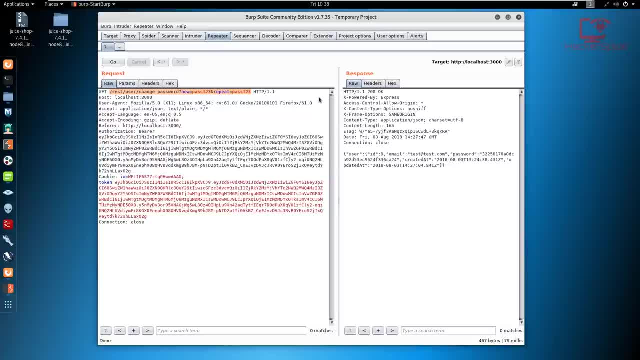 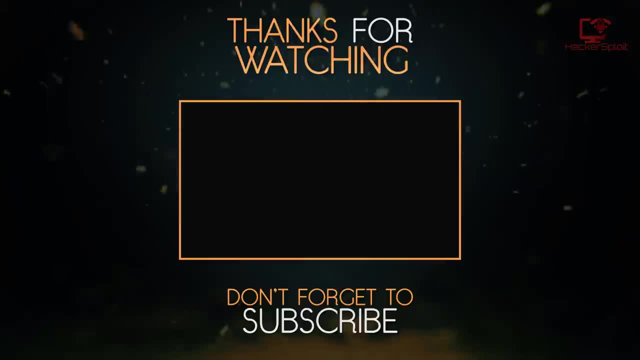 being said. that's going to be it for this video, guys, and I'll be seeing you in the next video. Peace. 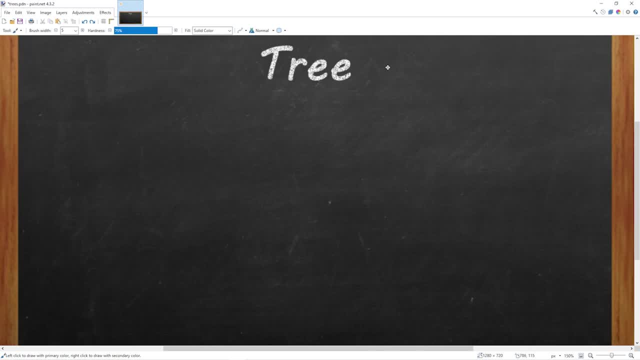 All right, everybody. Here's a quick introduction to trees. In this video we're only going to cover some of the terminology. A tree is a nonlinear data structure where nodes are organized in a hierarchy. This could be one example of a tree: It's made up of nodes and edges. Nodes could be: 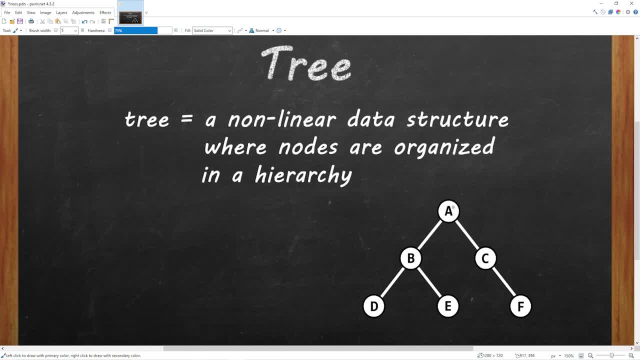 some piece of data and edges represent a relationship between two nodes. A real-life example of a tree could be a family tree. Maybe we're at node D, That's us, Or me Or you. B is a parent, E is your brother or sister, A is a grandparent, C could be an aunt or uncle And F? 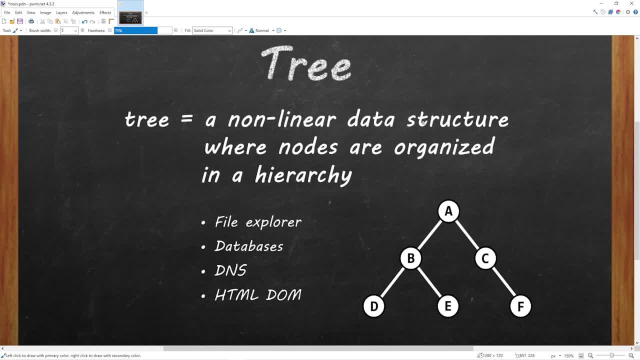 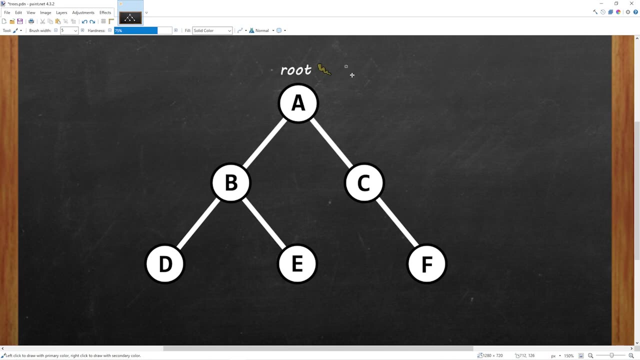 is your cousin. A few examples of where a tree data structure would be used in programming or technology would be file explorers, databases, domain name servers and the HTML document object model. The top of the tree is known as the root node. The root node doesn't have any incoming.